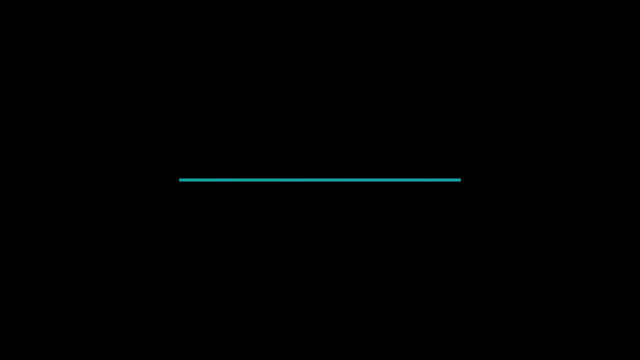 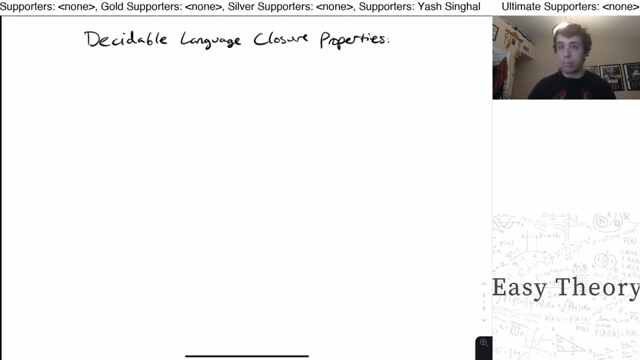 Hi and welcome back to another edition of Easy Theory. So today we're going to be looking at decidable language closure properties. So I get this question asked all the time: what are the closure properties for a particular class of languages? So we're going to be talking. 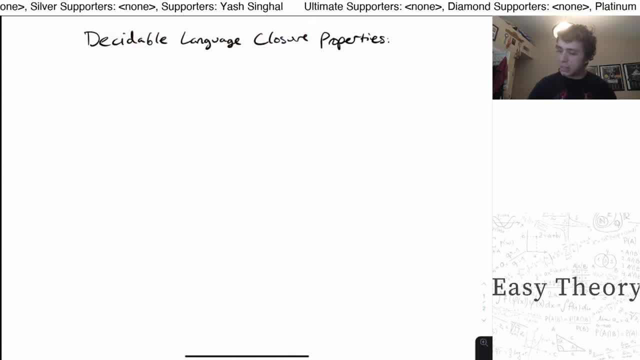 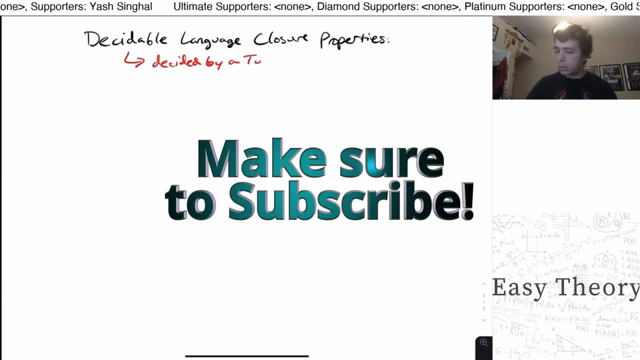 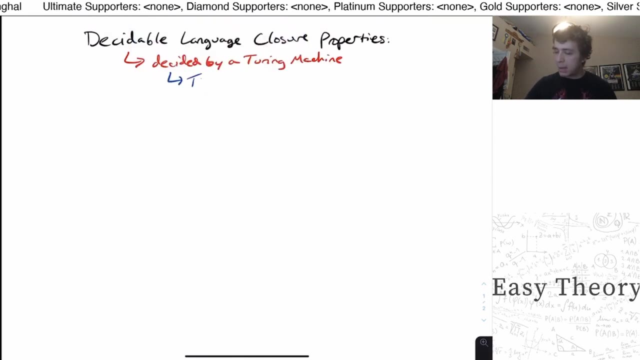 about the decidable languages today. So what is a decidable language? It's a language that is decided by a Turing machine. And what does decided mean? Decided means the TM runs, if I can spell, runs in a finite amount of time, regardless of what the input is. 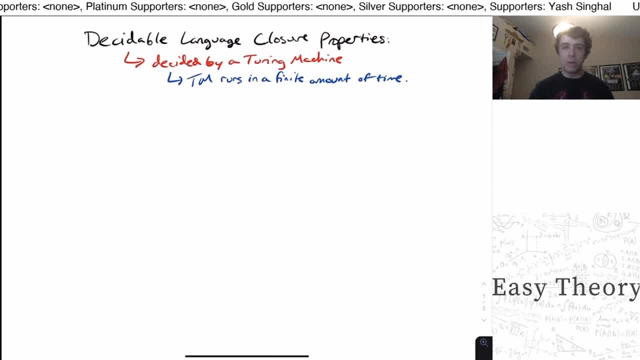 So if I give you any type of input and the Turing machine is a decider, it must say accept or reject in a finite amount of time. It can never run forever. There could be a Turing machine for this language that runs forever on the strings that are not in the language. That is called a recognizer. 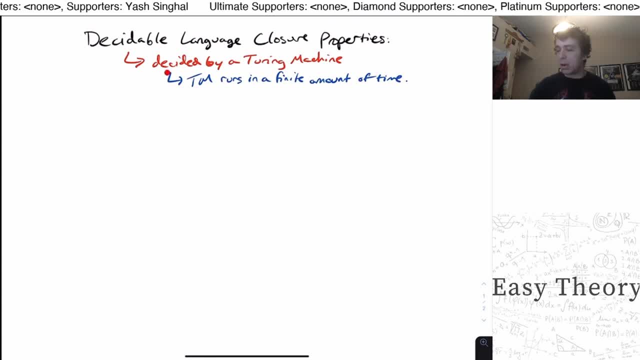 But here we're talking about Turing machines that are deciding the language. They always run in a finite amount of time, even for the strings, not in the language. So let's handle the main five operations. So the first one is complement. So if we have a Turing machine that runs for a finite amount of time, 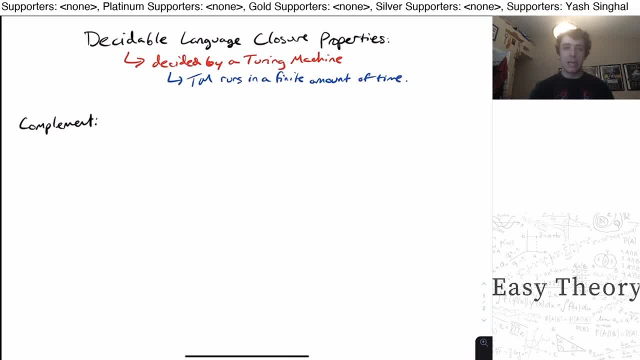 well, that means that it will hit the accept state or the reject state in a finite amount of time. So couldn't we just switch the role of the accept and reject state? And it turns out we can. So here let's just swap the Q accept state and the. 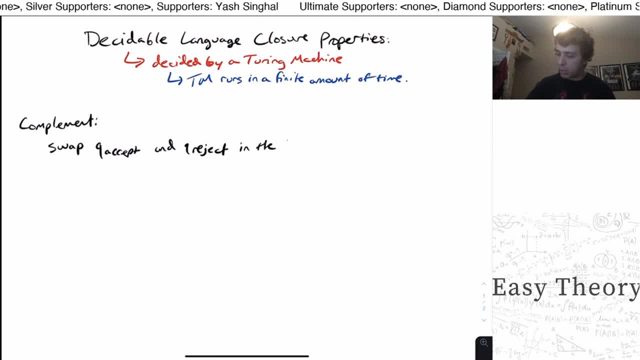 Q: reject state in the Turing machine. And we can do this because there's only one accept state and only one reject state in every Turing machine, or at least in this model of Turing machines. And we are allowed to do this because, well, if it hits the accept state before in a finite amount, 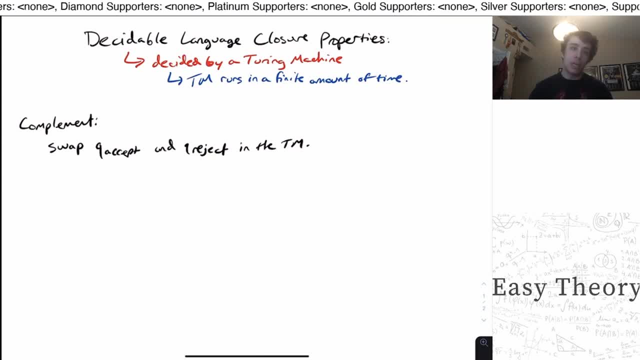 of time, then in the modified machine it hits reject in a finite amount of time and vice versa. So this doesn't work with rects, It doesn't work with recognizers, because if it hits the accept state in a finite amount of time, 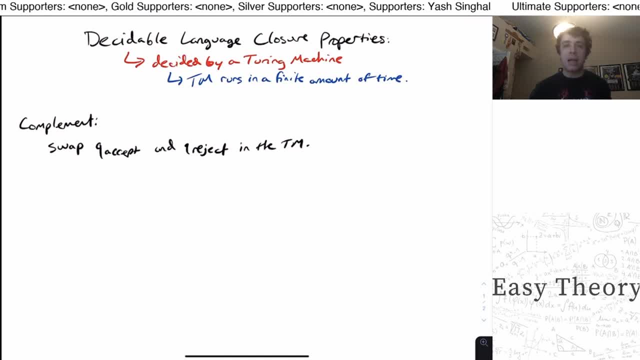 it hits the reject state in a finite amount of time, but not the other way around. If it hits the reject state, then it will hit the accept state. But what if it runs forever? Well, that means it was implicitly rejected, the string, But now we need to accept it. 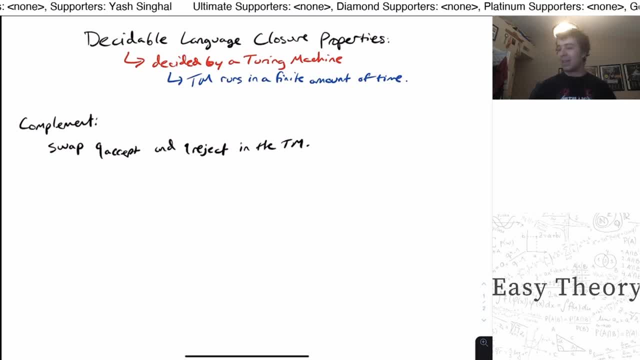 which means we need to run in a finite amount of time. So it doesn't work for recognizers. And it turns out that there is no Turing machine that runs for a finite amount of time. So it doesn't work for recognizers. So it doesn't work for Turing machines. 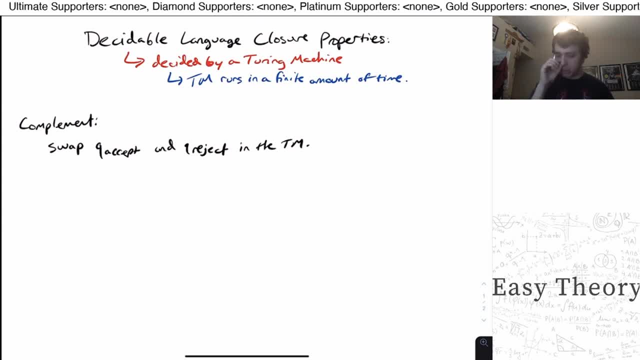 We need to run a Turing machine for the complement of some recognizable languages. But for decidable we can, because we guarantee to hit one of the two states in a finite amount of time, regardless of what the input is, And so by swapping them we can guarantee. 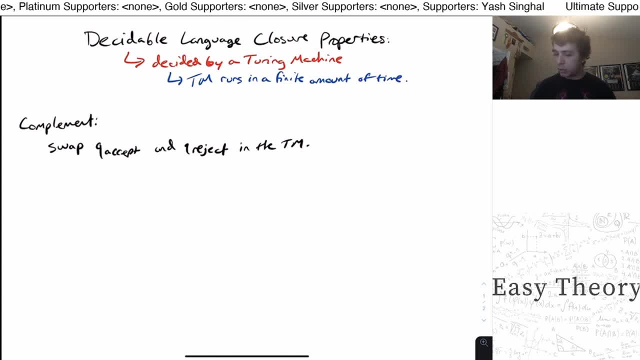 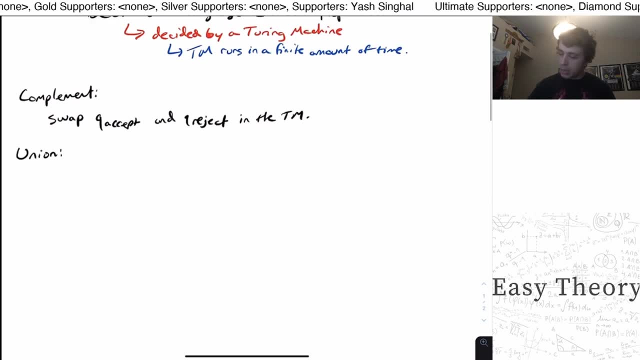 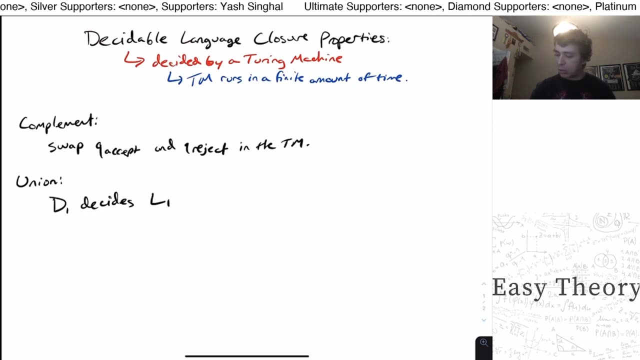 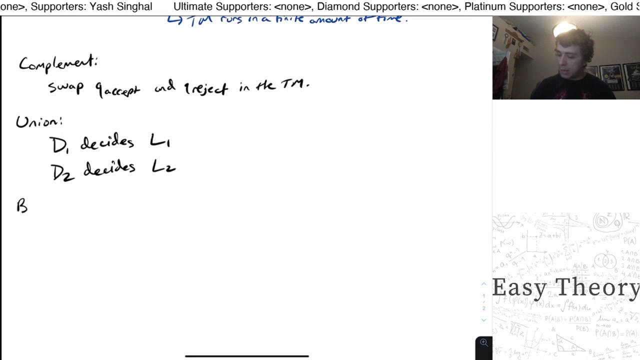 the same thing about the complement language, And so the modified Turing machine gets the complement here. Okay, what about for union? Well, here this is asking: if D1, is a Turing machine that decides language, L1,, D2 decides L2.. Well then, how do we build a decider? 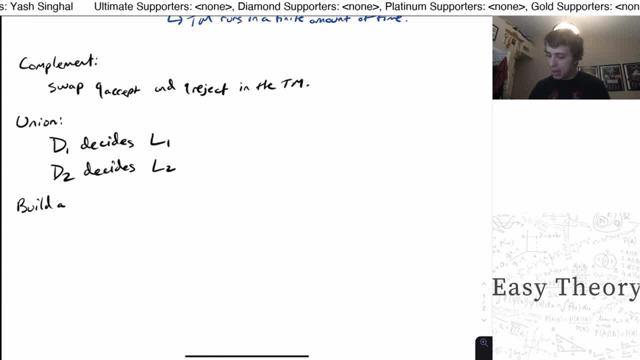 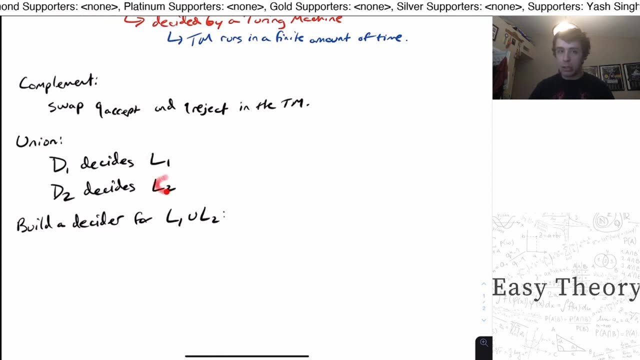 for I can't spell decider, build a decider for the union of the two languages. Well, how do we do this? Well, that means that we're given a string and we want to figure out whether it's in the language L1 or in the language L2.. So we can actually just query the two Turing. 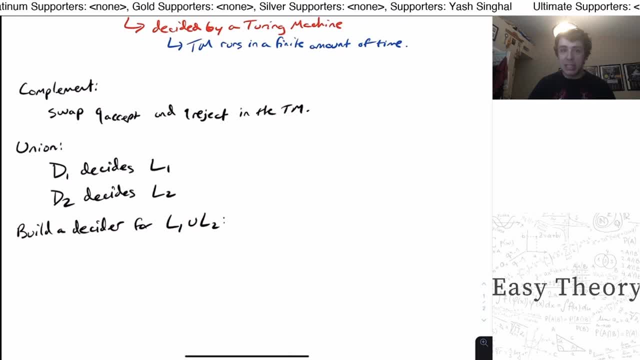 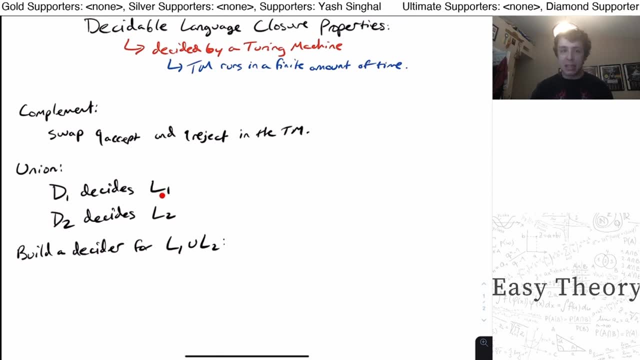 machines here and just ask: does this machine accept it? And that is fine, because each of these two machines decides the language and so they run in a finite amount of time. So what we can do is just say, okay, well, let's run that string on this machine and run that string on this machine. 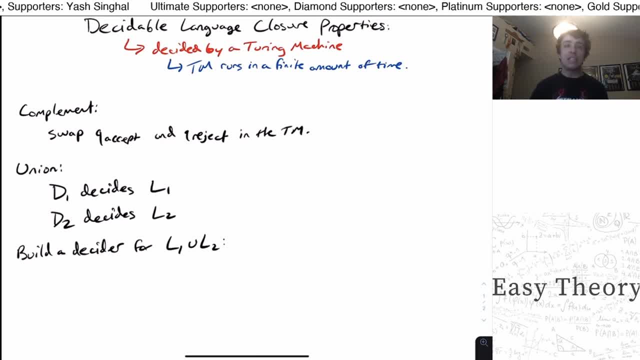 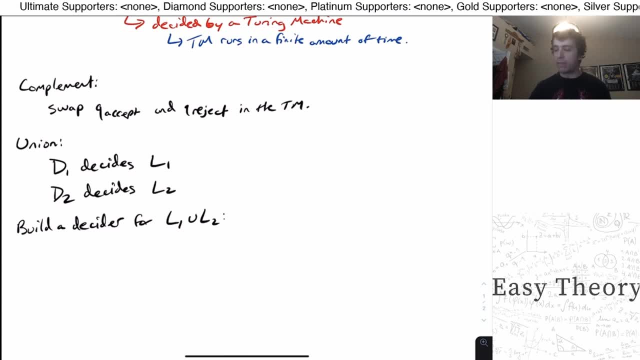 and we accept ourselves If at least one of the two accepts, because if either one of them accepts, then it must be in the union of the languages. So how do we build a decider? So it's going to be over here. On input W, let's run D1 on W, then run D2 on W. 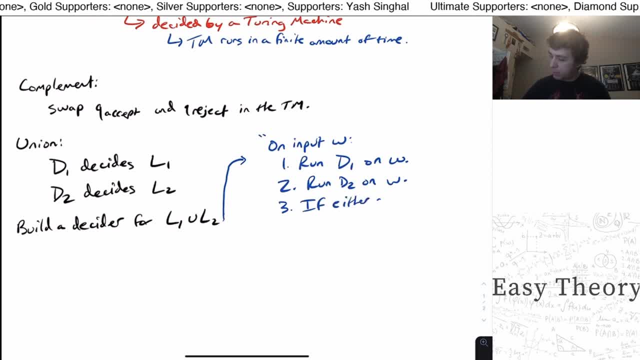 And if either accepts, then we accept and we can reach this step in a finite amount of time, because the first two steps run in a finite amount of time, And otherwise we reject, because if neither one accepts, then it can't possibly be in the union. So we reject here And we could have 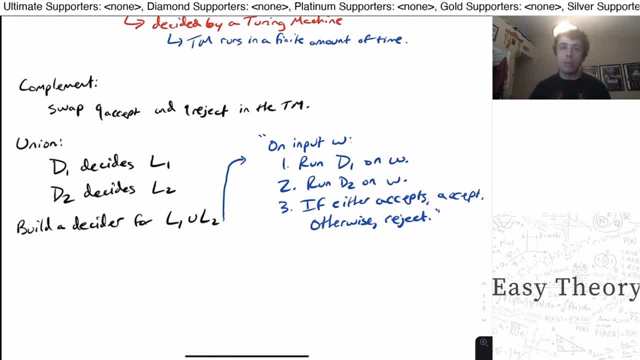 accomplished the same thing with complement. We can just run the one machine on W and then just invert the answer. That's totally fine too. So this runs in a finite amount of time, Pretty clearly. What about for intersection? Well, for intersection, well, isn't it kind of the same thing as union? 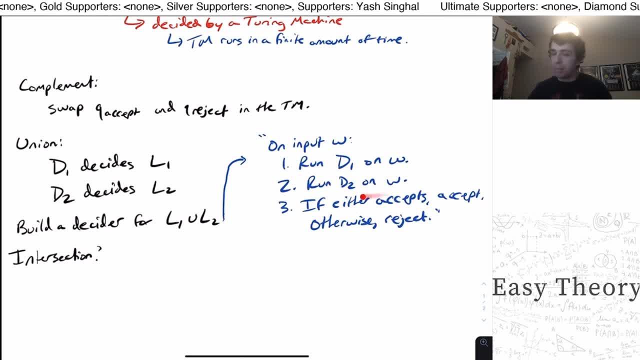 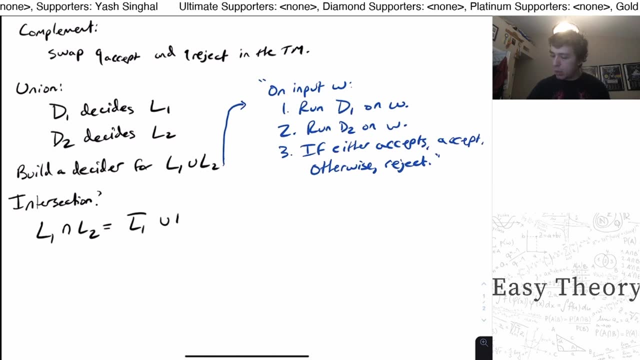 Except that we require this condition to be: if both of them accept, then accept. But another way to view it is: we can actually just use De Morgan's laws, So the intersection of two languages is always equal to the union of the complement languages, and then complement the whole thing. well, since we showed that, 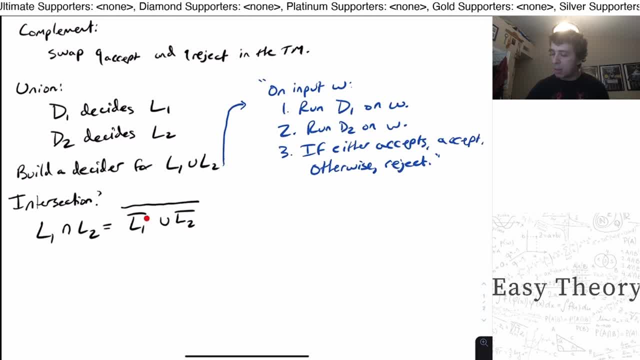 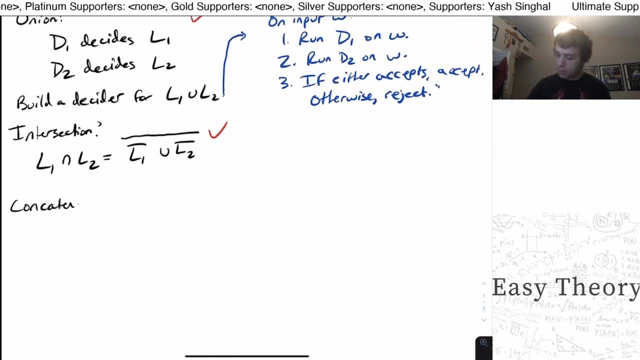 decidable languages are closed under union and complement, and these are a finite number of both of them. therefore, they're closed under intersection two. so this one is yes, yes, yes. what about for concatenation? so this is: we're given a string, W, which is the characters 0, 1 through through WN, let's say, and we want: 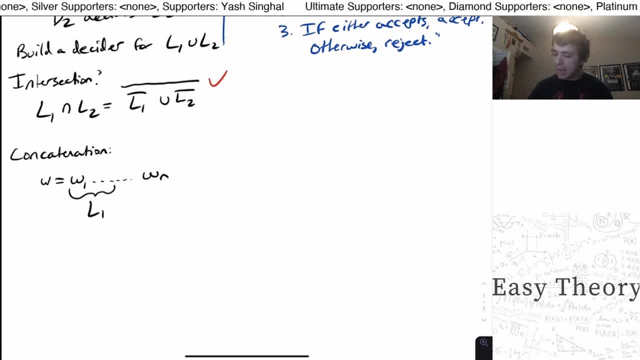 to figure out if there is some kind of split where the first half is from the first language and the second half is from the second language. we'll note that if the split is here, then there are only finitely many possible splits into two pieces, so the split could be at the beginning or after the first character. 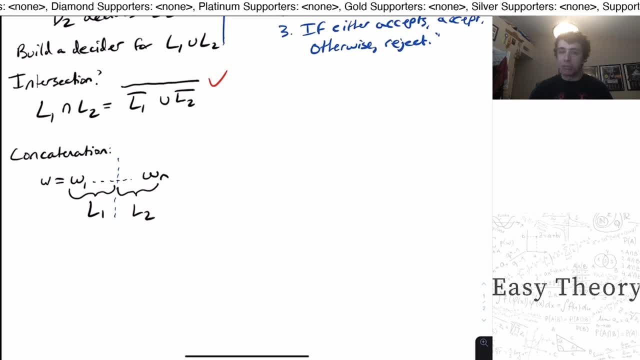 or after the second, except for the first character, or all the way after the last one. so how do we build a decider for this? on input W. what we need to do is split W into two pieces in all possible ways, and we can do that because the length of the input is always finite, so there are only a finite. 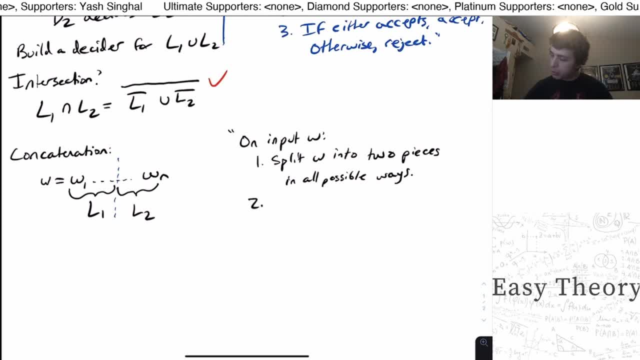 number of splits that we need to actually check. so then run the first machine, D 1 on the first piece and D 2 on the second. but here we, instead of having either one except, we need to have both of them. except because we need the first machine to accept the first part and the second machine to accept the 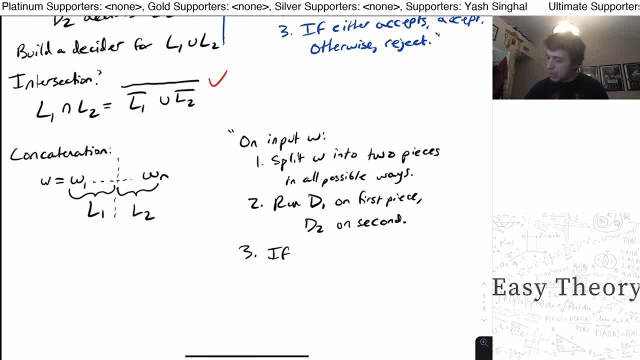 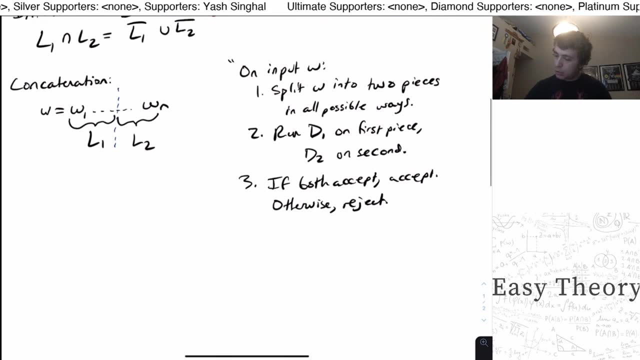 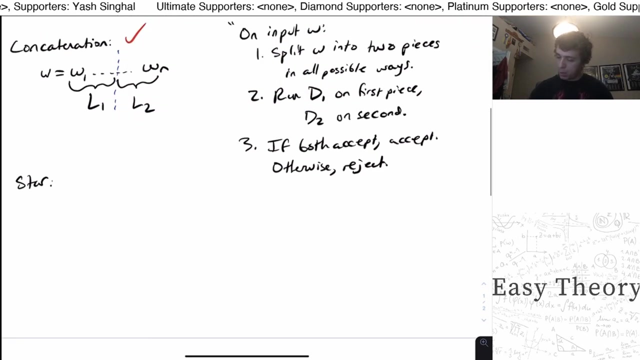 second part. so if these two machines both accept, then we accept ourselves. you should always accept yourself, otherwise reject. so then now, what about star though? and I should mark that this is check. what about for star? well, that's just saying that if we again have our input, 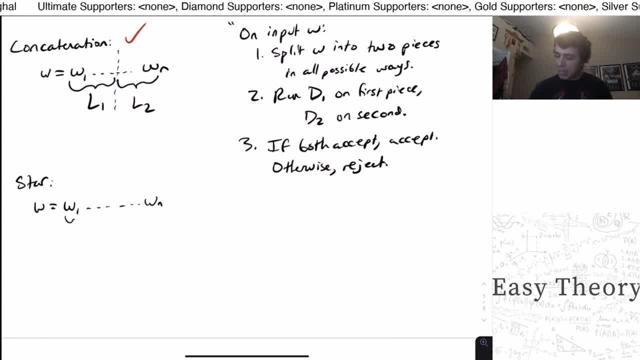 W1 and Wn. Well, this is asking if we can split it some number of times, maybe four or maybe possibly more, where each piece comes from that one language. So remember, the stars only apply to one language, not two. So let's just say that the language here we're looking at is L1, just as an example. 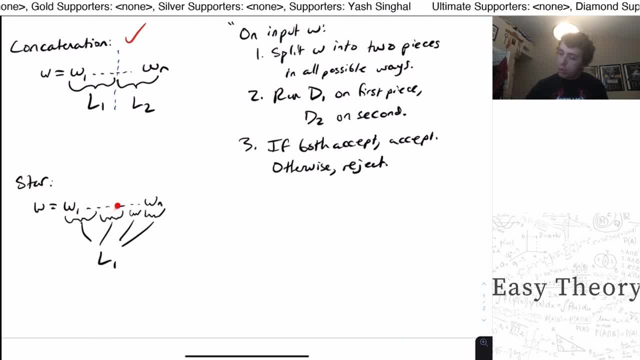 So how do we actually do this? Well, note that there are only finitely many possible splits here. Well then you may say: okay, well, what if one of the splits is empty and the other one's empty at some other point? 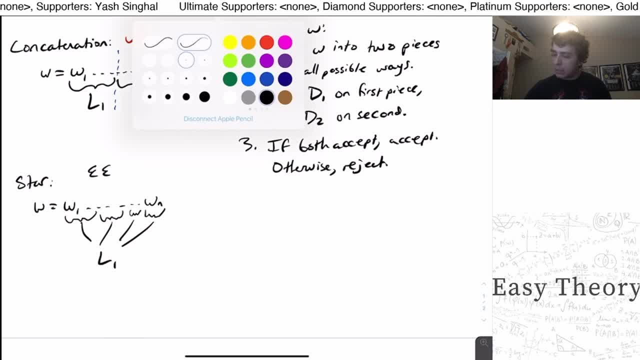 Well, here, what we can do is let's just ignore the case of where we have two of the pieces being empty. One of the pieces can be empty, but not the other one and not another one, And we could, if we didn't check that, have the case of where we have so many pieces. 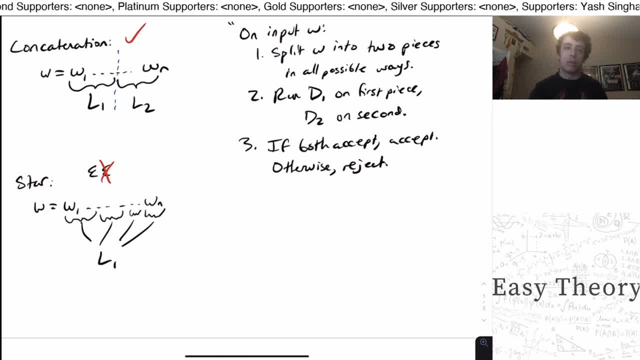 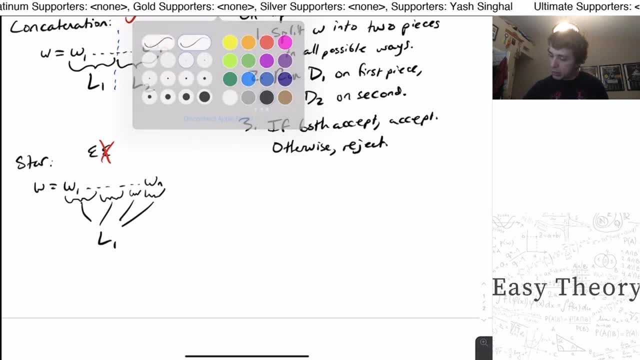 we have infinitely many choices of the empty string, which is not something that we would be able to check in a finite amount of time, So what we need to do for a decider, then, is very similar. On input W: split W into any number of pieces in all possible ways. 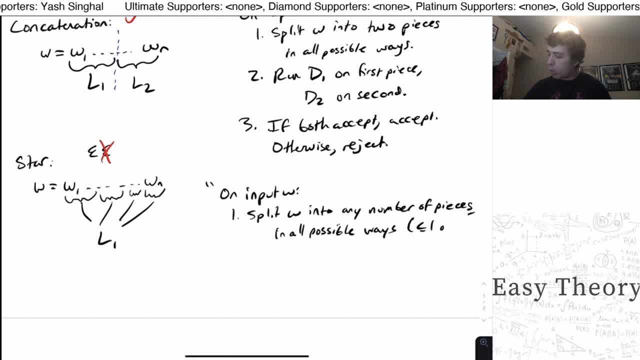 and have at most one of the pieces being the empty string, And there are only finitely many of them. So then let's run the first, the machine corresponding to this language- L1, on each of the pieces, So we'll just run all of them.